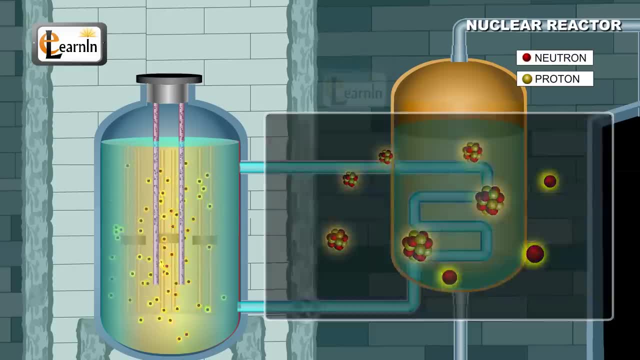 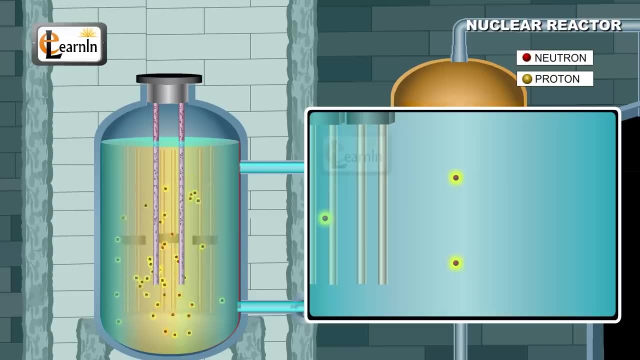 This is where a moderator is extremely useful. Moderators have the capability to slow down, or in other words, moderate the speeds of these high energy neutrons so that they can in turn be used for a chain reaction to trigger multiple fission reactions of other uranium-235 nuclei. 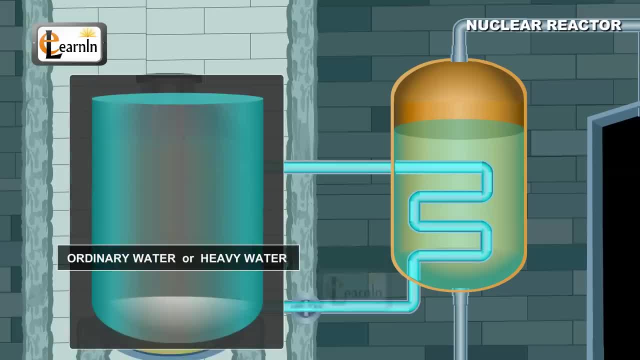 Commonly ordinary or heavy water is used as a moderator in nuclear reactors because of the deuterons present in them, which are capable of producing fission reactions. This is where a moderator is extremely useful. Moderators have the capability to slow down, or in other words, 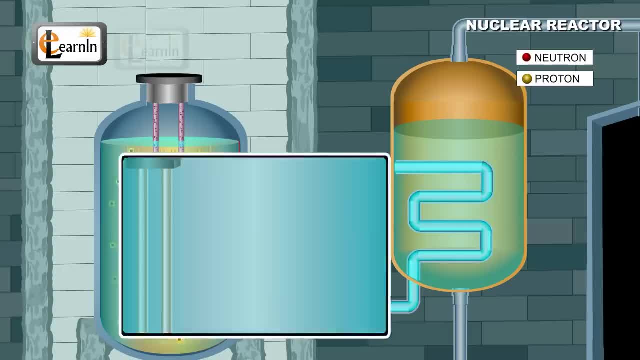 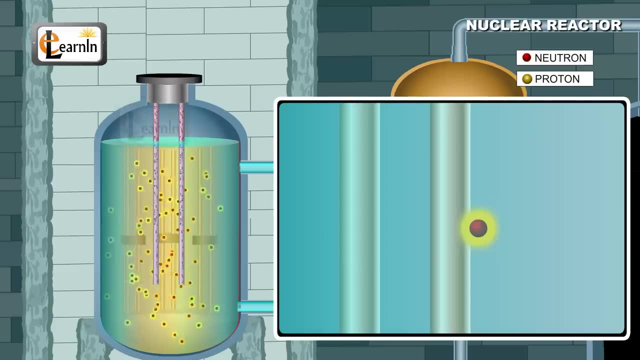 moderate the speeds of these high energy neutrons so that they can in turn be used for a chain reaction to trigger multiple fission reactions of other uranium-235 nuclei Water molecules in a moderator are useful in slowing down the high energy neutrons which leave the fuel element after nuclear fission. These high energy neutrons collide. 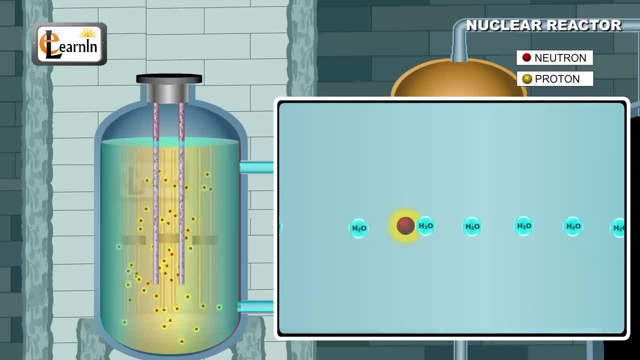 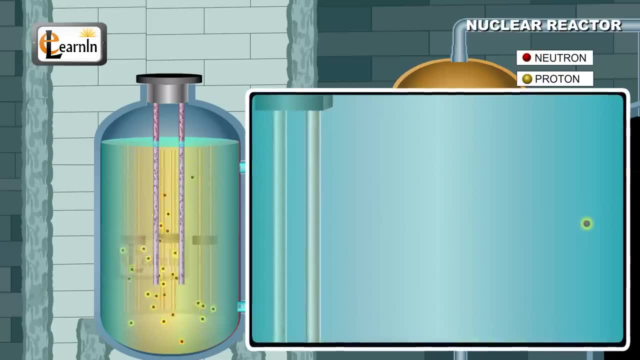 with water molecules, thereby losing out on some energy with every collision and therefore slowing down substantially. A new fission reaction can now be triggered using this slow neutron by striking it with the fuel element. The third and most prominent part of a nuclear fission reaction is: 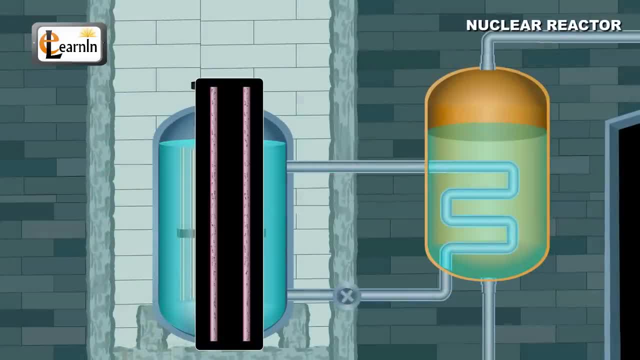 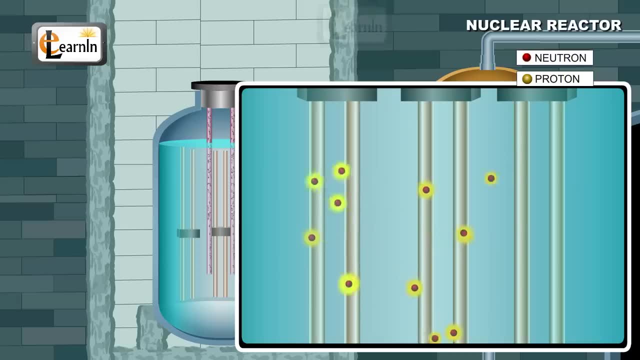 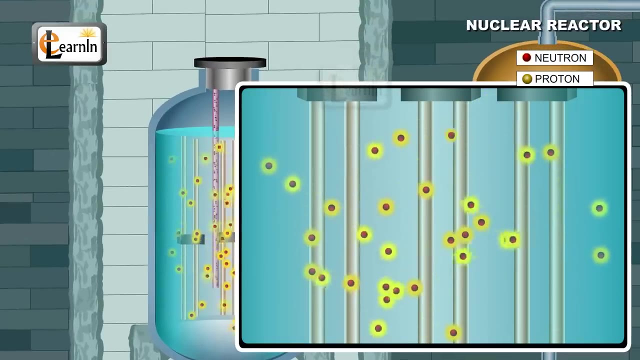 the control rods. In order to get a steady output of energy from the nuclear reactor, every single fission reaction should trigger another fission reaction and ensure the availability of spare neutrons released to trigger the chain reactions. By controlling the number of spare neutrons available at any given time, the rate of nuclear fission chain 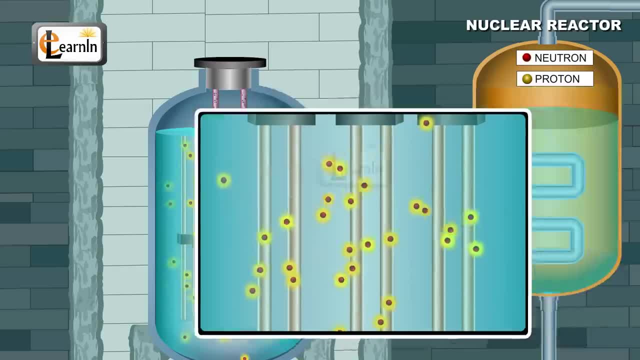 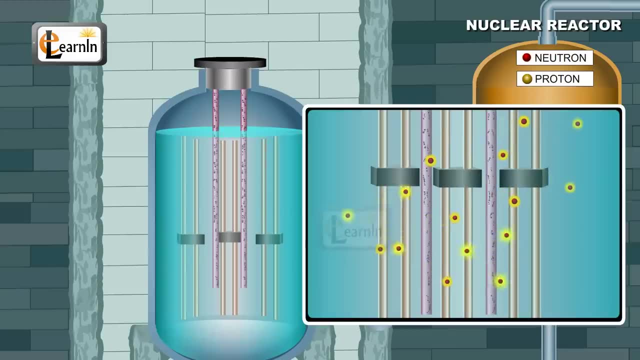 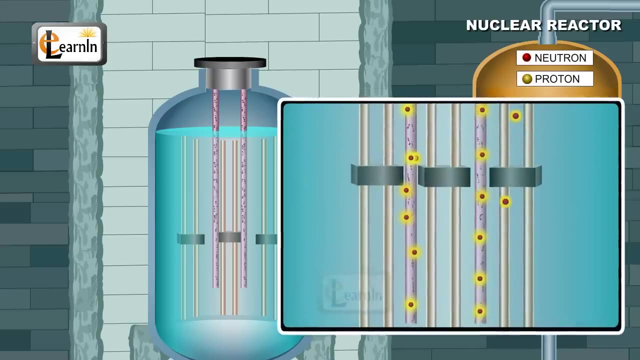 reactions can be controlled. This control on the fission reaction can be maintained using control rods. The main function of the control rods is to absorb any excess or spare neutron in the moderator in order to prevent any further fission reactions. Usually, such control rods are made of boron or cadmium. 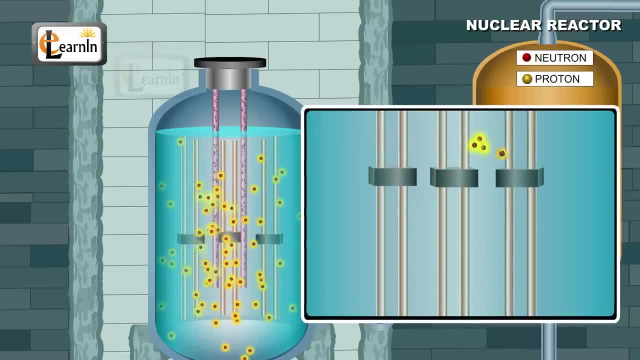 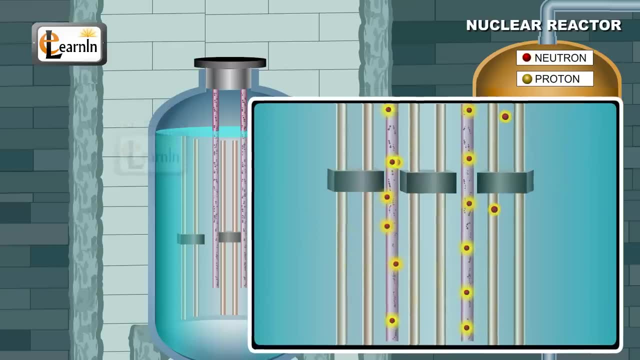 To increase the rate of fission reactions. these rods can be removed from the moderator. A steady output of energy can thus be maintained by inserting or removing the control rod. A steady output of energy can thus be maintained by inserting or removing the control rod. 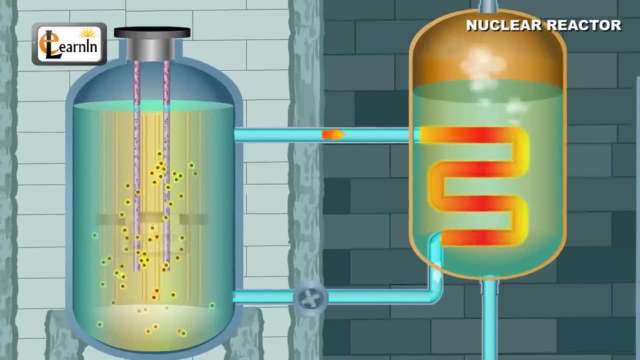 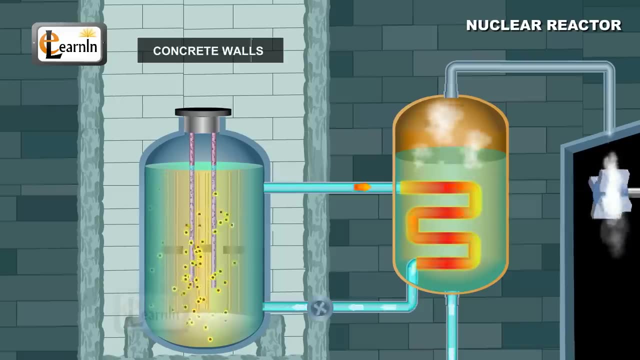 A steady output of energy can thus be maintained by inserting or removing the control rod. Now that we know the components of a nuclear reactor, let's understand the working of a nuclear reactor. It's usually enclosed in a shield made of thick concrete walls.